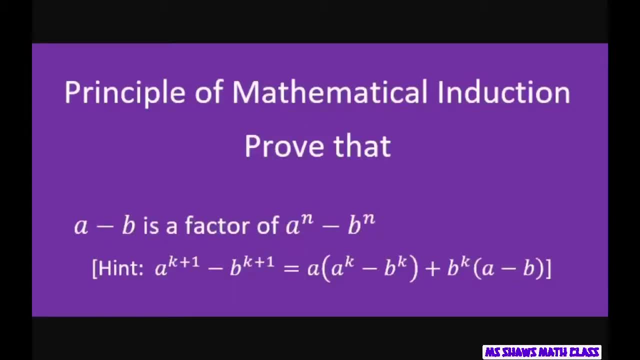 Hi everyone. we're going to use the principle of mathematical induction to prove that a minus b is a factor of a to the nth power minus b to the nth power. Before we get started, remember that let's just do a squared minus b. squared That equals a minus b times a plus b. 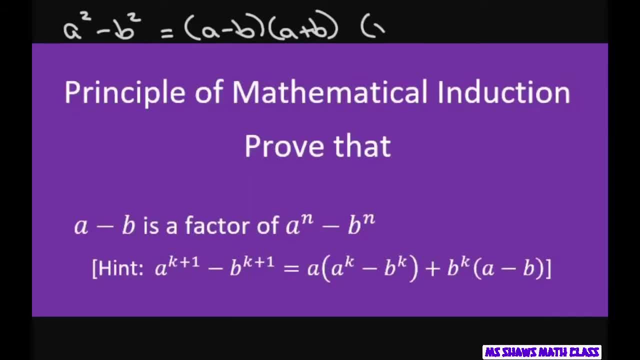 So let's just look at if I had x squared minus 4, that's going to be x minus 2 times x plus 2.. Now for that. if you FOIL this out, I'm going to go back. this way- you would get x squared minus 2x plus 2x plus 2 squared. 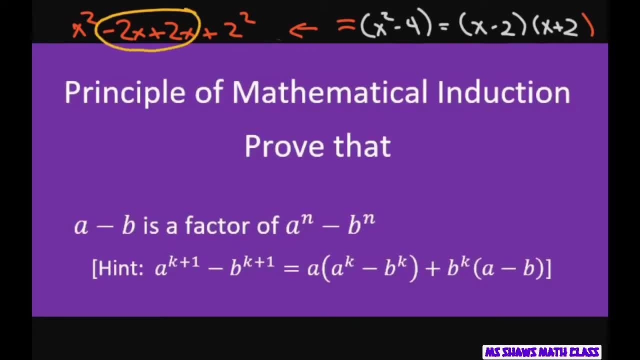 And you notice how these two terms go away. This is a square. This is a square. This is minus, sorry, minus 2 squared, And that's where you get back to that. So we're going to expand our binomial using this procedure, but without any numbers. 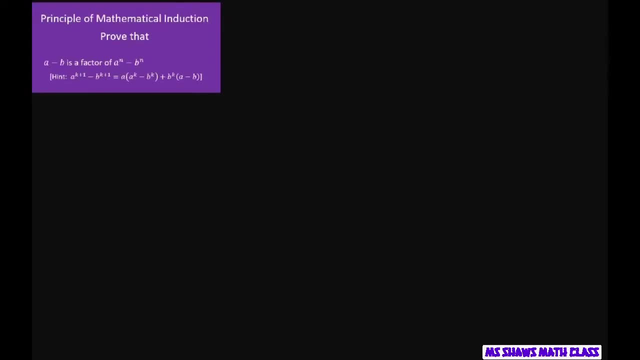 Alright, so we'll get started. So our condition 1 is to show that it works for n equals 1.. So a minus b is a factor. So our condition 1 is to show that it works for n equals 1.. If a minus b is a factor of a to the k power, minus b to the k power, then we're going to show that a minus b is a factor of a to the k plus 1, minus b to the k plus 1.. 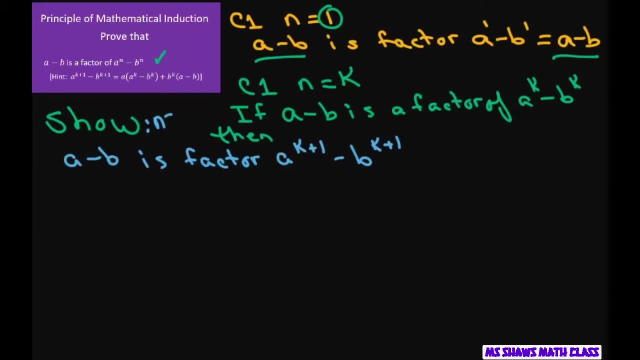 So we're showing n equals k plus 1.. Alright, now this is where we're going to get to where I was talking about earlier. So this expanding this, this is a to the k times a. That's what this is.